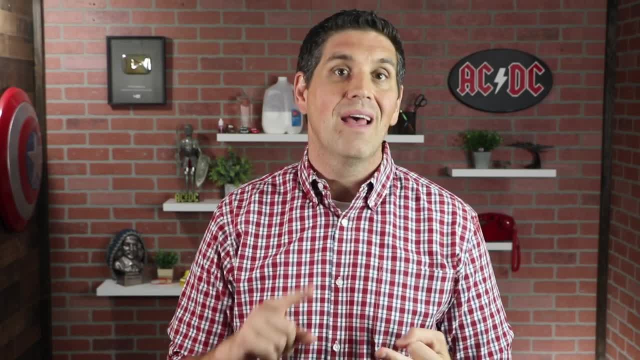 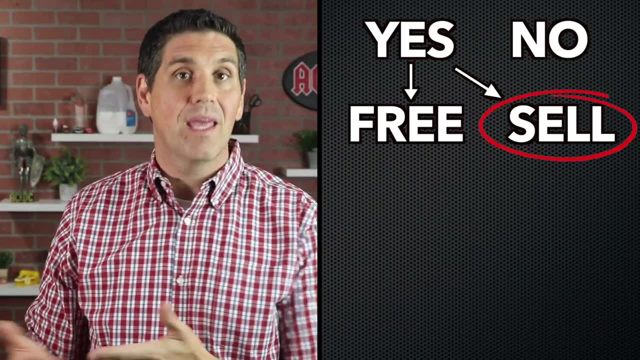 So the explicit costs of getting a haircut and going to the post office and mailing out the hair and the implicit costs of my time and my energy. And if I ask him for any money at all, that means I'm just selling him my hair. 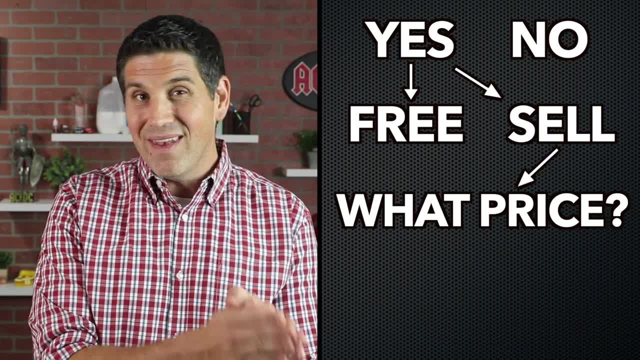 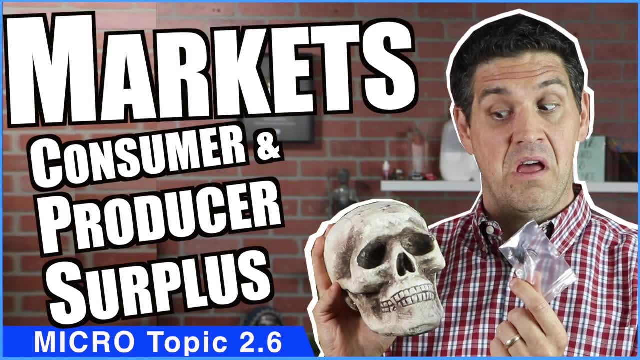 So I have to figure out what price to charge to him and maybe the next person that asks for my hair, which means I have to be able to understand and analyze a market. The market demand curve that you learn about in econ is actually made up of individuals. 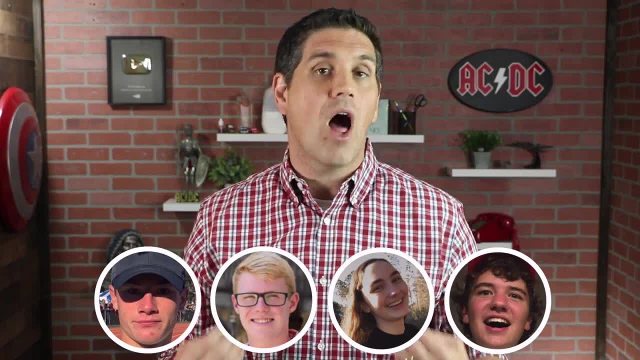 For example, let's say there's four students and they're all interested in getting a lock of my hair. So let's say the price is $100.. The only person who would pay that much is Sam. He'd be willing to buy one. 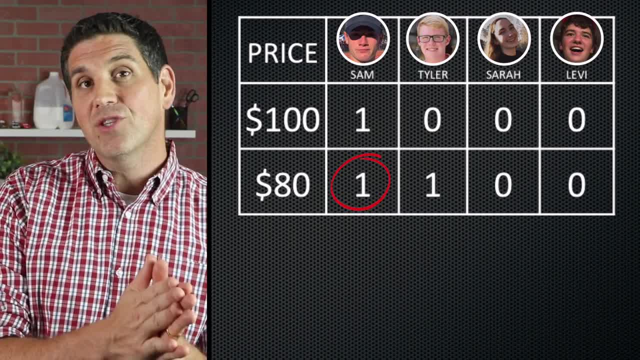 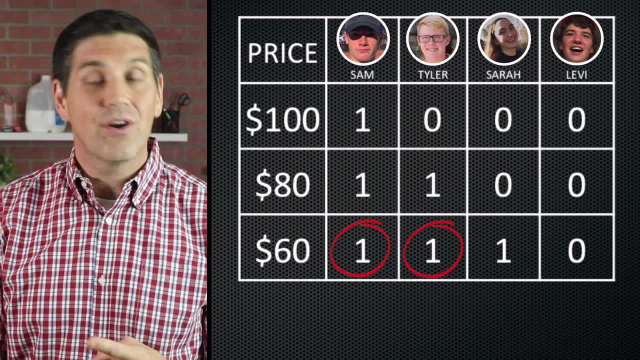 Now, if the price falls down to 80, then he'd still be willing to pay, but so would Tyler. So there'd be two people who wanna buy my hair, And if the price fell even further down to $60, then Sam Tyler and Sarah would all wanna buy one unit. 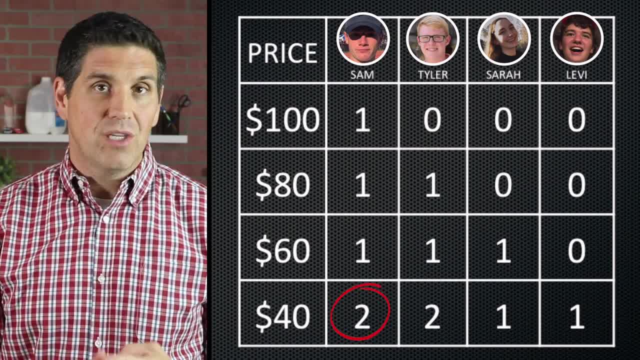 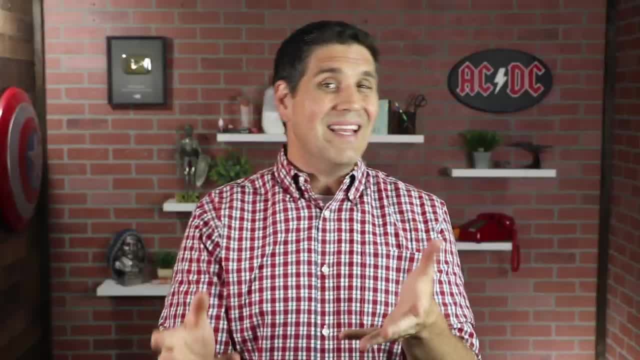 And if the price fell all the way down to 40, then Sam would buy two, Tyler would buy two, Sarah would buy one and this new person, Levi, would also wanna buy one. You get the idea. People are different. 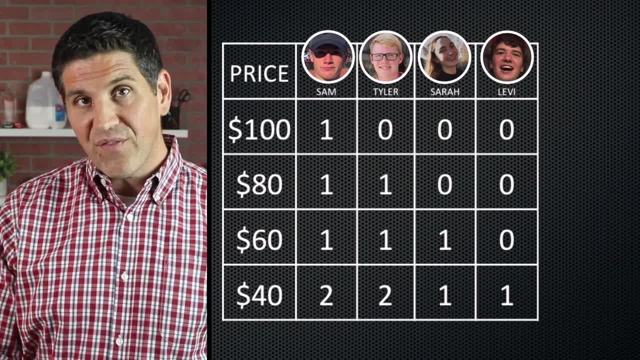 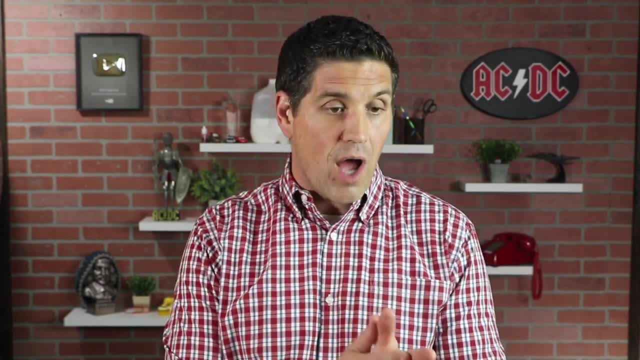 so they have a different willingness to pay. When you add up all these individual preferences, you get the market demand and can draw a downsloping market demand curve. And the market supply curve is created the same way. It's based on the cost and preferences of individual sellers. 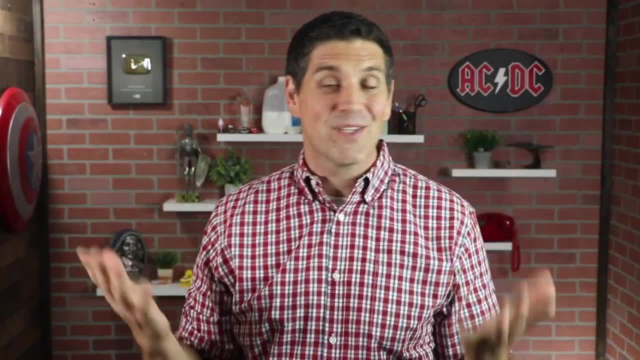 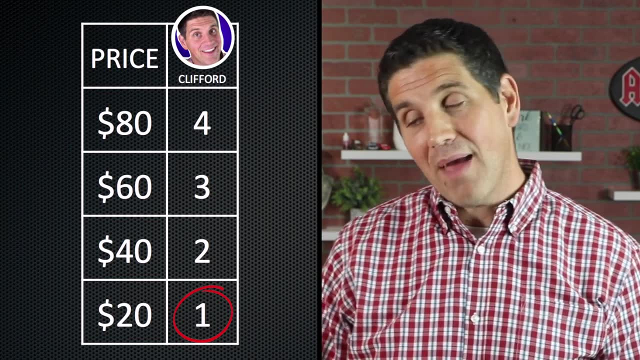 Now, in this case I'm the only supplier of Clifford hair. but the same principles apply: If the price is anything below $20 and it's just not worth it, it doesn't cover my opportunity cost. If the price was $20, maybe I'd just sell one just for fun. 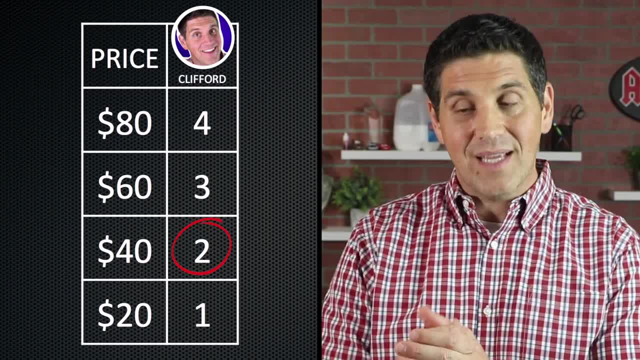 but if the price goes up to 40,, I'd sell two. If it goes up to 60, I'll sell three, and if it goes up to 80, then I'd sell four locks of my hair. Notice as price increases. 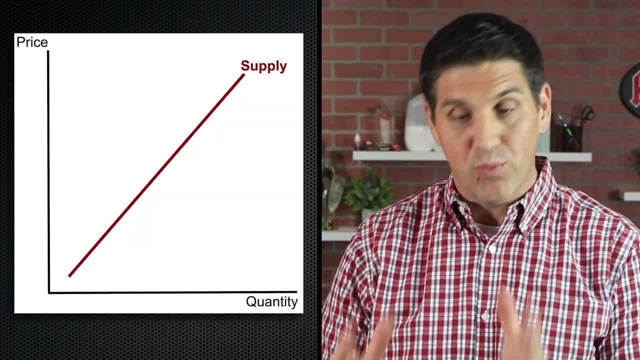 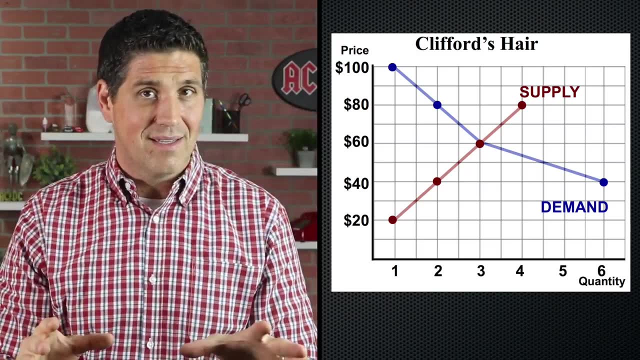 individual producers have an incentive to bring more products to the market, which results in an upward-sloping supply curve. When you put the supply with the demand, you get equilibrium. that's easy. You learn that in your class. But what you probably haven't thought about, 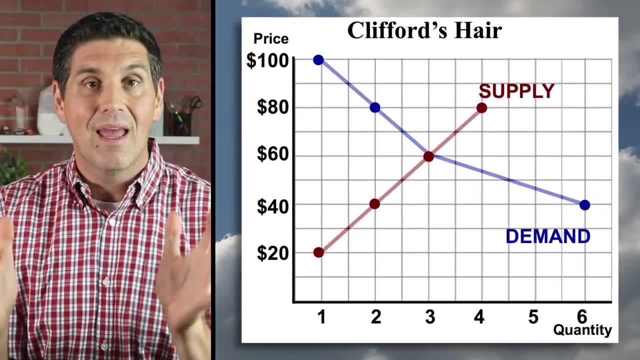 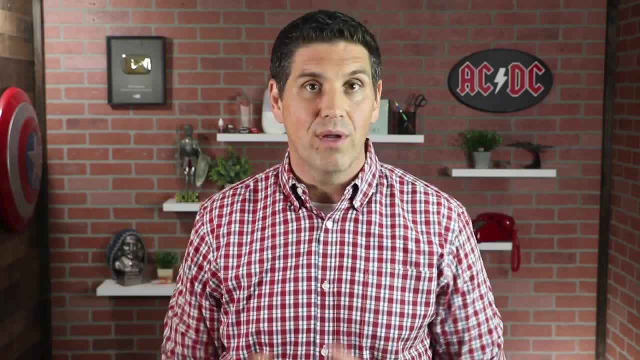 is how ingenious the supply is, How ingenious and amazing this is for organizing society and distributing our scarce resources. Imagine instead that there wasn't a market and I randomly gave out locks of my hair to random students. The chances that I would pick the exact students. 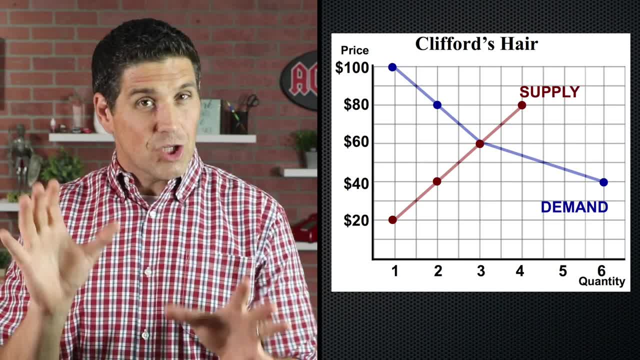 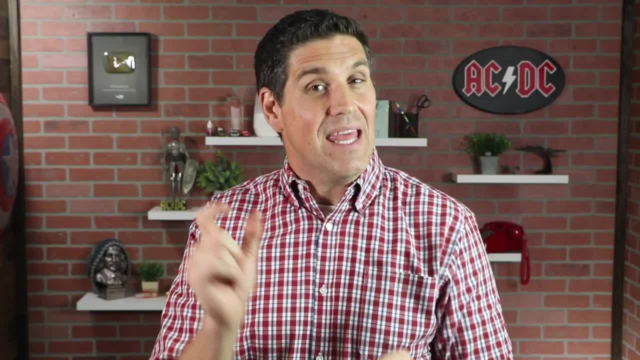 that want my hair the most is pretty low, but a market solves that problem. Markets cause goods and services to flow to the consumers that want them the most and they prevent the inefficient use of our resources. You might not think that's a big deal. 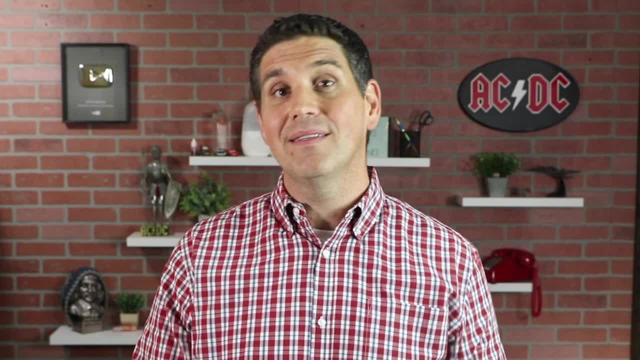 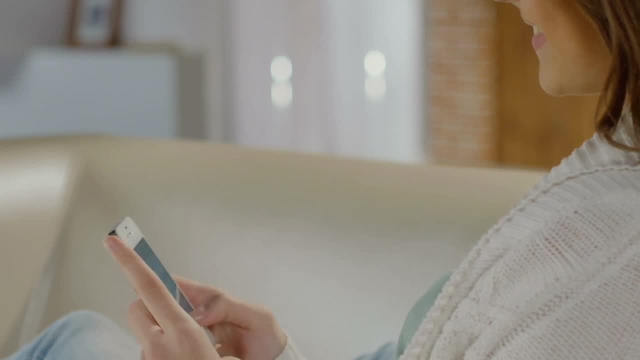 but I'm telling you it's like the biggest deal. Everything around you right now exists because of this market system: Your phone or your computer, that you're watching this video on YouTube itself, your clothes, your house- all this stuff exists because supply and demand. 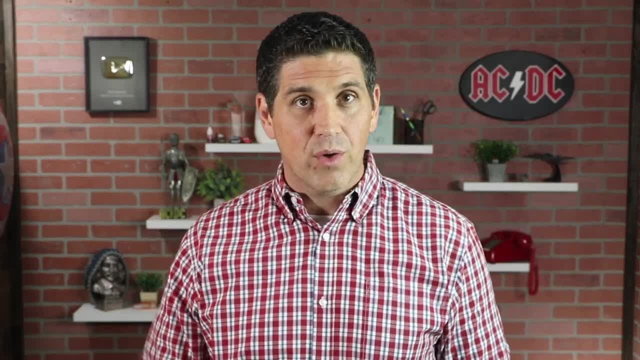 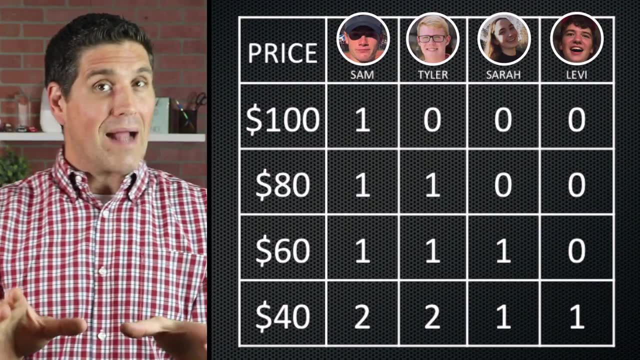 allocated resources toward their production. If there was an endless supply of resources, then we wouldn't actually need markets. Every person would just get everything they want. but Now let's go back to the numbers. Do you remember Levi? He was willing to pay $40 for a lock of hair. 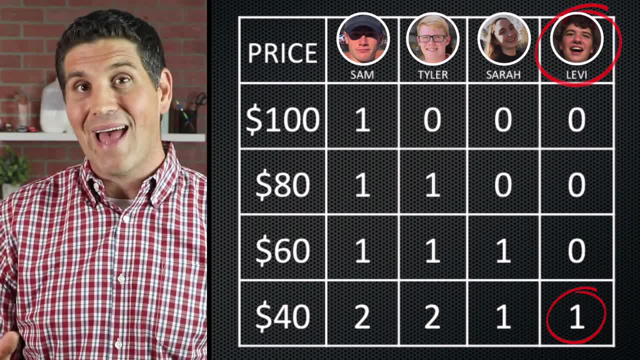 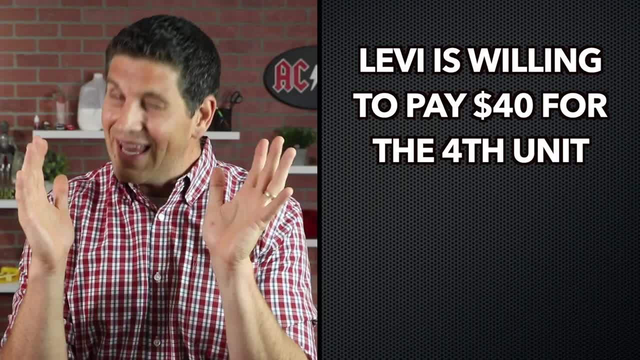 but he doesn't get a lock and you might feel bad for him, but if somebody's gonna miss out because of scarcity, it's best that it's him. He values the hair the least. In fact, if he got one, that would be extremely inefficient. 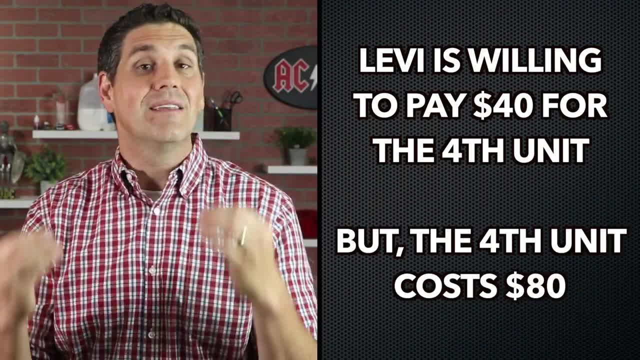 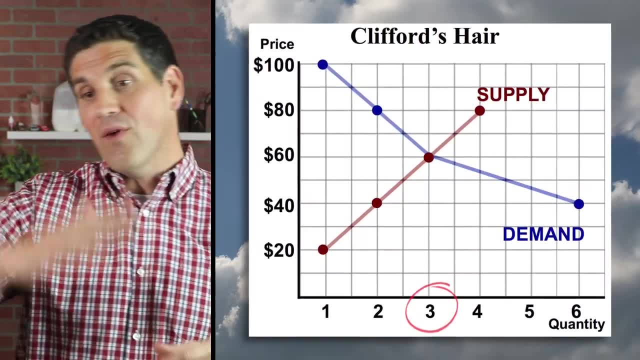 because the value he places on it- that $40- is less than my opportunity cost of producing the fourth unit. In other words, markets tell producers exactly how much to produce so they don't over-allocate resources towards things that people don't really value. 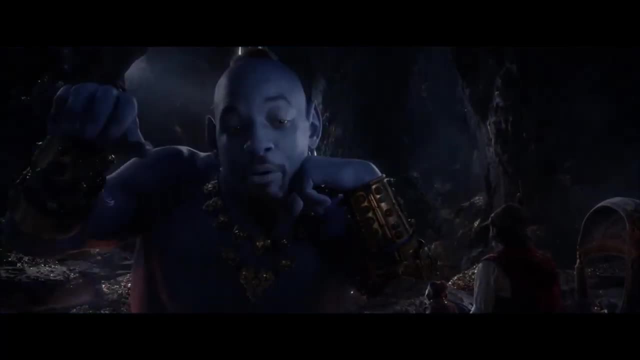 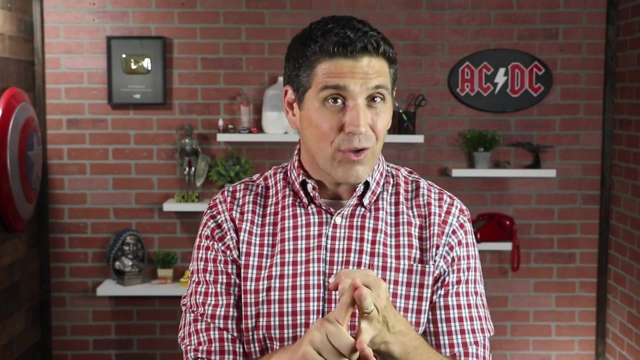 which is amazing. Markets are awesome. You can clap now In your standard microeconomics class. you have to be able to take this a step further and identify and calculate consumer and producer surplus. Remember that Sam was willing to pay $100 for a lock of hair, but he didn't pay 100. 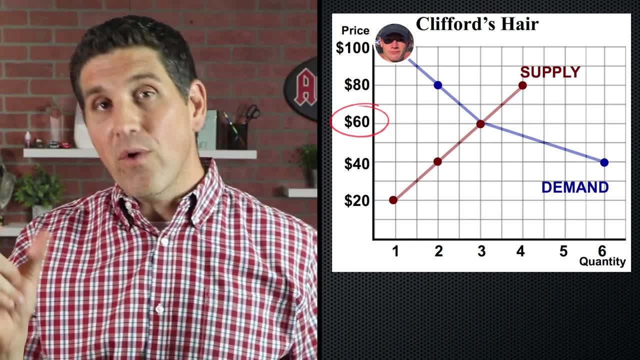 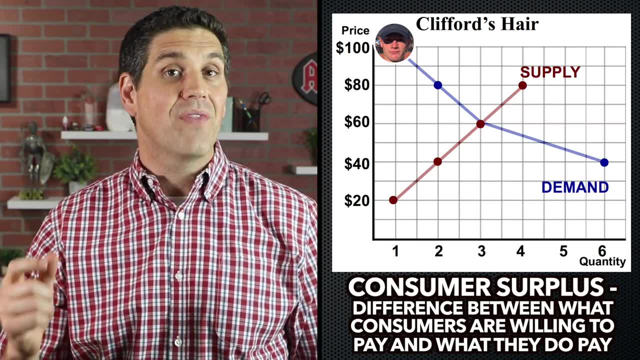 He paid the market equilibrium of 60.. The difference that- $40, is Sam's consumer surplus. It's the difference between what individual consumers are willing to pay for a good or a service and what they do pay, and it's not just Sam. 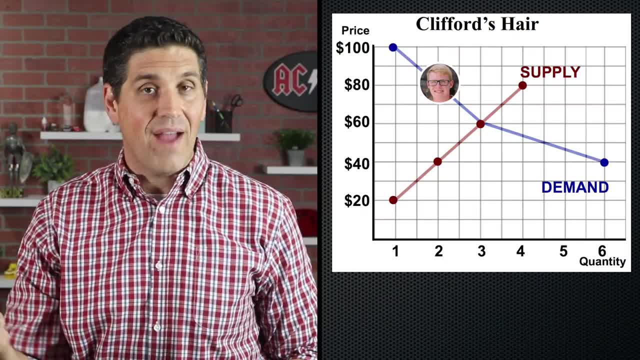 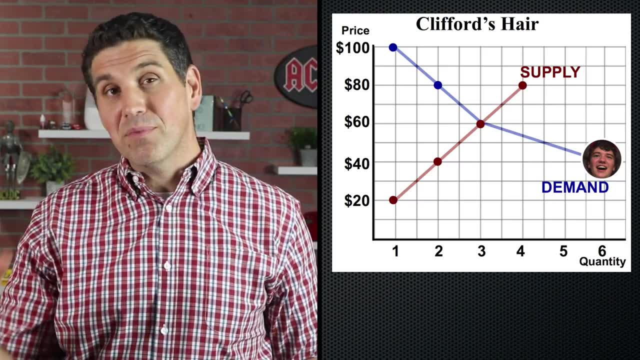 It's also Tyler, Remember. he's willing to pay up to $80 for the lock of hair, but he didn't pay 80. He paid 60, so that $20 is Tyler's consumer surplus. Now, Levi, he was willing to pay up to $40. 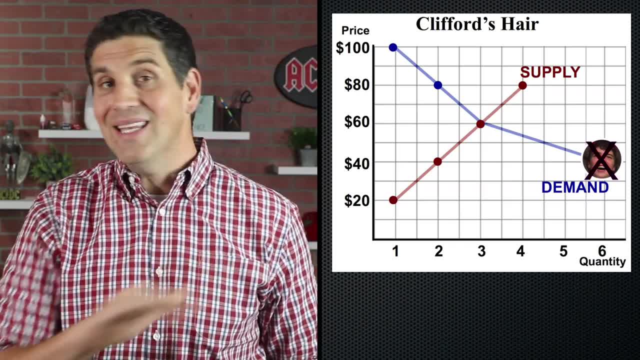 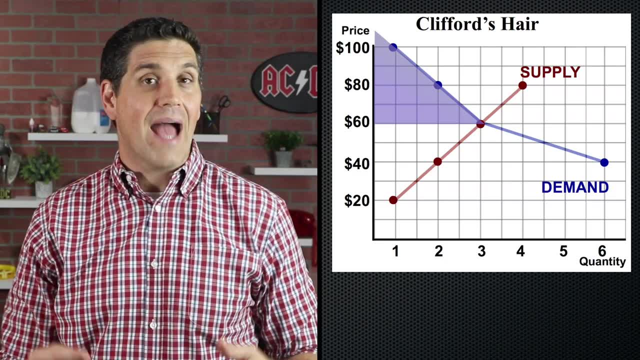 for a lock of hair and the market equilibrium price was 60,. so he didn't get the product. He gets no consumer surplus. Graphically, the consumer surplus is this triangle right here and in some classes you have to actually calculate it. 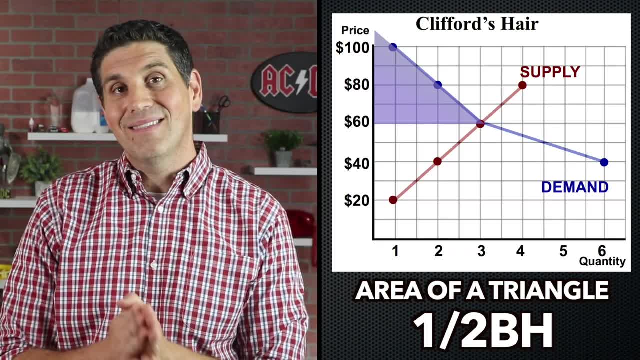 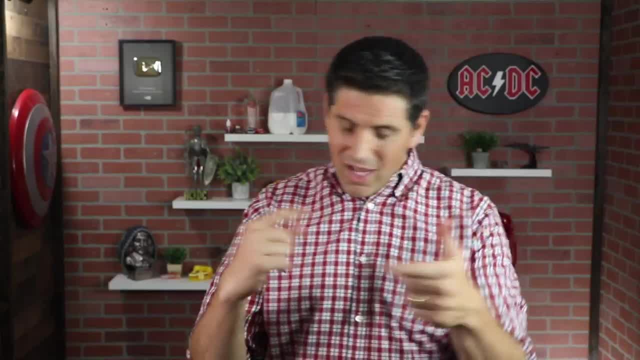 so remember it's just the area of a triangle 1 1⁄2 base times height. In this case the base is three units and the height is $40, so the consumer surplus is $60.. I know I covered that quick. 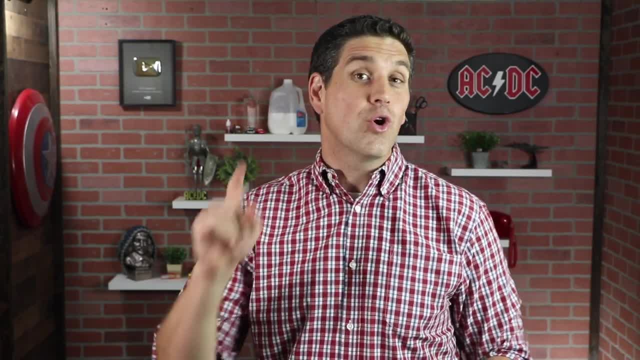 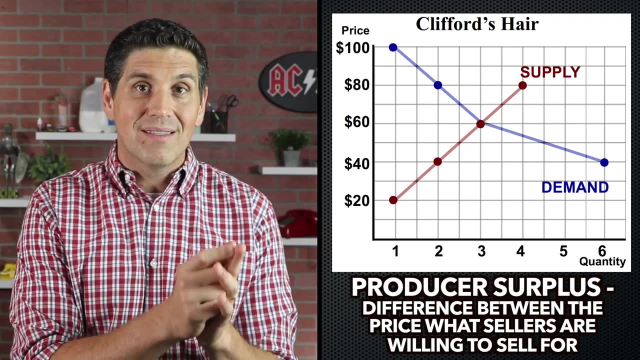 Make sure to watch the end of the video where I give you some practice multiple choice questions so you can do those calculations. Producer surplus is the exact same idea, except we're looking at seller. so it's the difference between the price and how much a seller is willing to sell a product for. 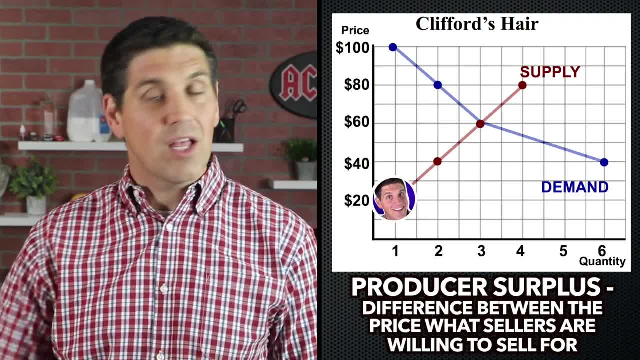 For example, I'm willing to sell the very first lock of hair for $20, but I didn't sell it for 20.. I sold it for the market price of 60,, so that $40, that difference is my producer surplus. 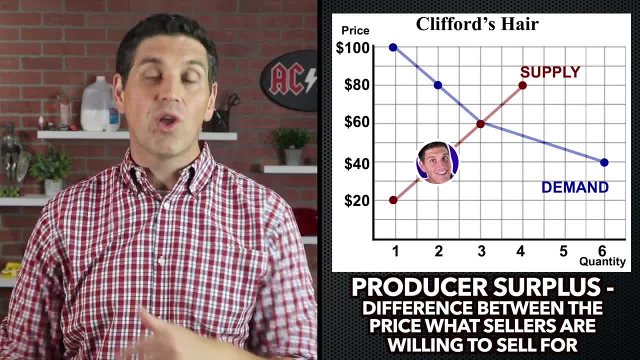 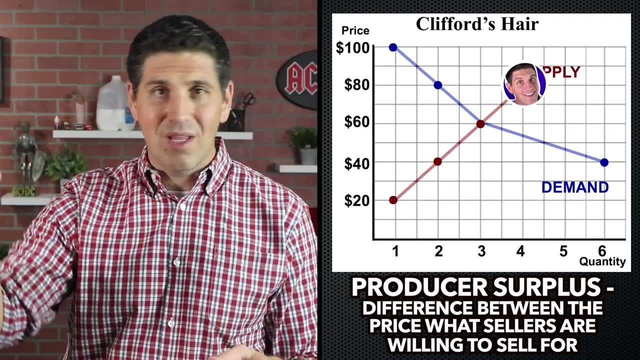 for that first unit. For the second unit, I was willing to sell it for $40, but I sold it for 60, so that $20 is my producer surplus. for the second unit. What about the fourth unit that I had a super high opportunity cost. 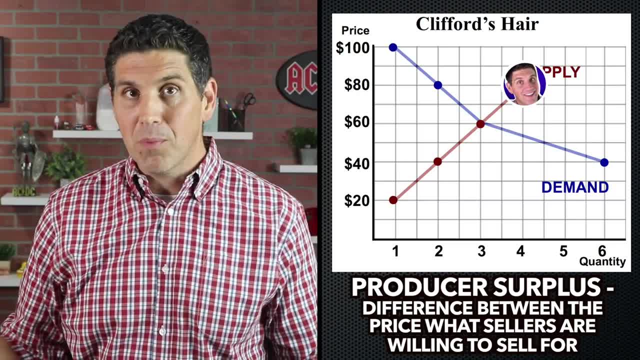 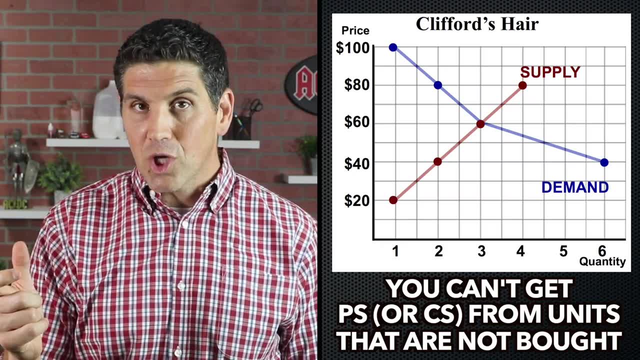 you had to pay me a lot to go sell the fourth unit. Where's the producer surplus? There is none. I wasn't actually able to sell that unit. So just remember: you can't get producer surplus or consumer surplus from units that were never bought or sold. 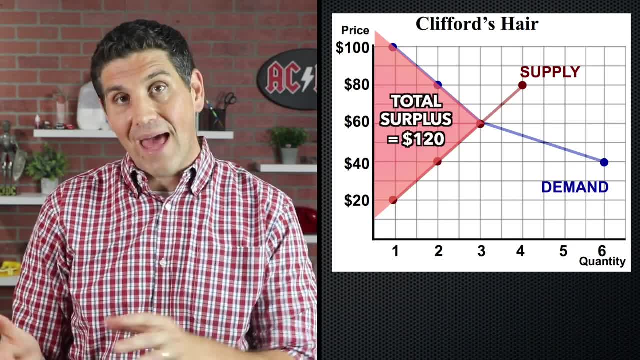 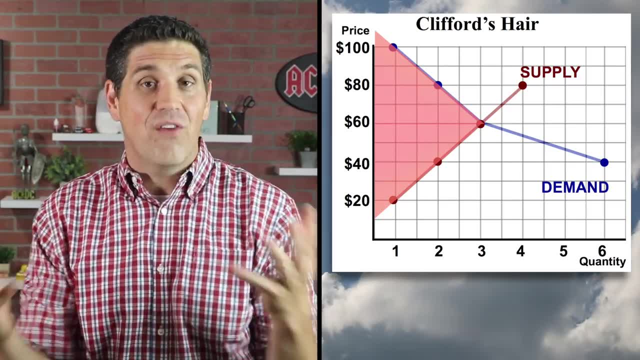 The actual area of producer surplus is this triangle down here, And together consumer surplus and producer surplus make up this area, which is total surplus. And this shows why markets are so darn efficient. They allow as many buyers and sellers as possible to benefit from voluntary transactions. 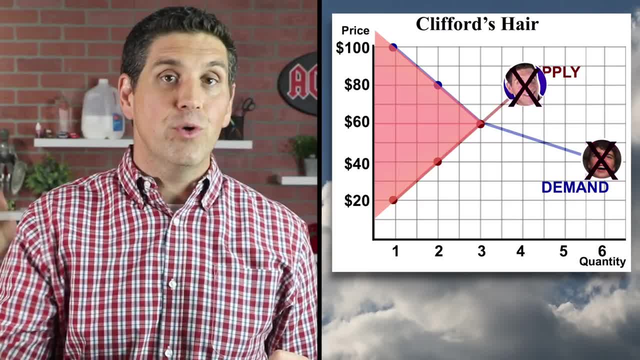 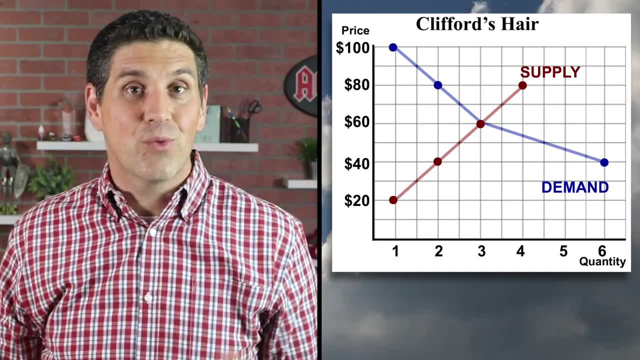 People who don't really want the product don't get it, and high-cost producers that have a high opportunity cost don't sell it. It's a super efficient way to organize society and distribute scarce resources. For example, let's say I produce only one lock of hair. 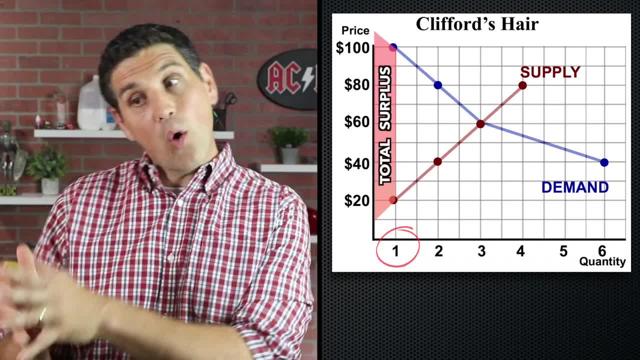 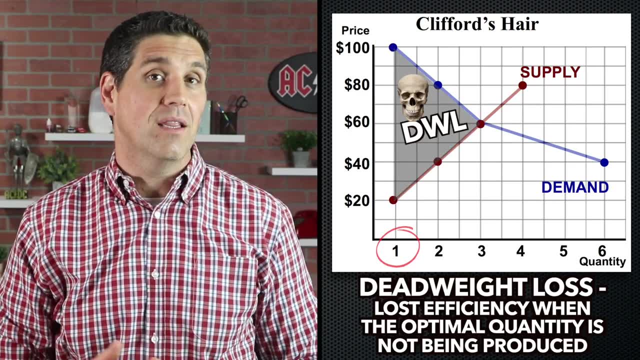 This isn't efficient because there's lost consumer and producer surplus, or total surplus is less. Economists have a really cool name for this lost efficiency: when you're producing the wrong output, It's called deadweight loss. Trust me, you're gonna see it over and over again. 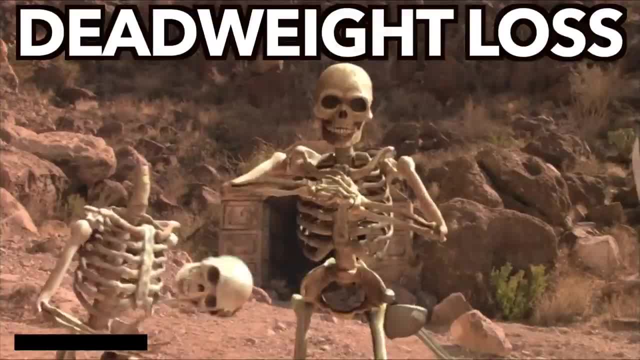 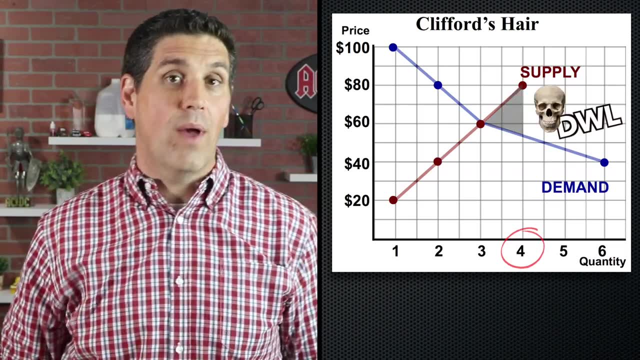 in a microeconomics class, You have to be able to identify it and calculate it. So don't be afraid. This is the cost of deadweight loss. Let's look at the other side. Let's say I produce four units. That too would be inefficient and cause deadweight loss. 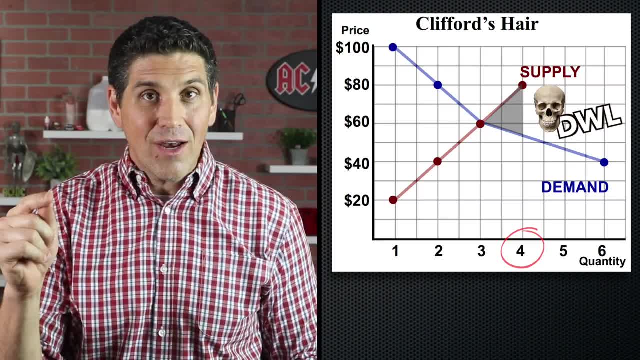 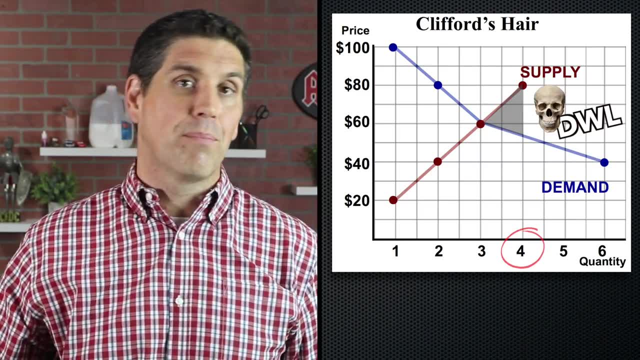 The reason why is because the cost of producing that fourth unit is greater than what society's willing to pay for it. So the market's saying: don't put your resources in producing more hair. Society doesn't want this. Stop producing, produce less. 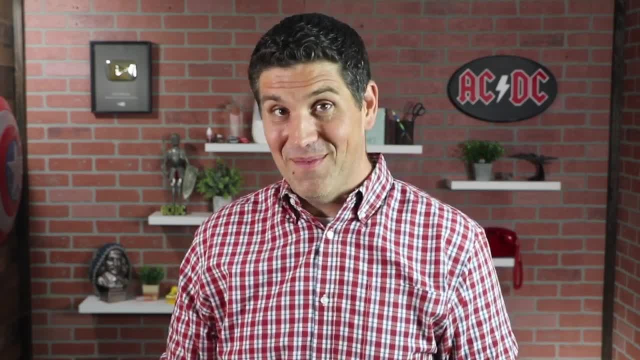 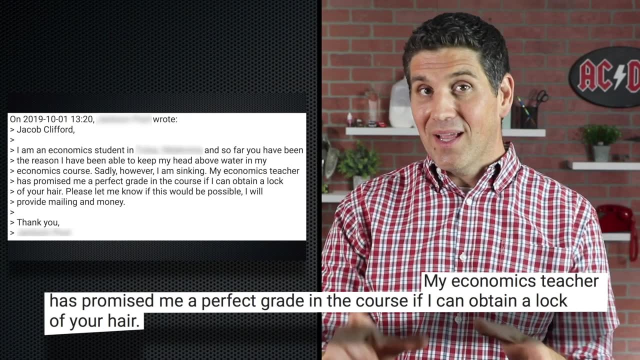 I'm sorry I get all geeked out on this, but markets are awesome, but except when they're not. There's a detail I left out from the email from the guy who wanted my hair. Reason why was because his teacher said he'd give him. 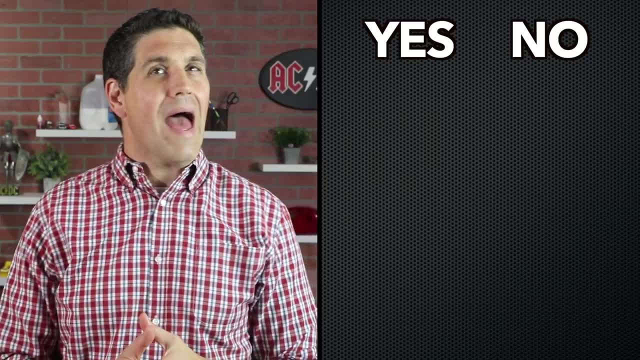 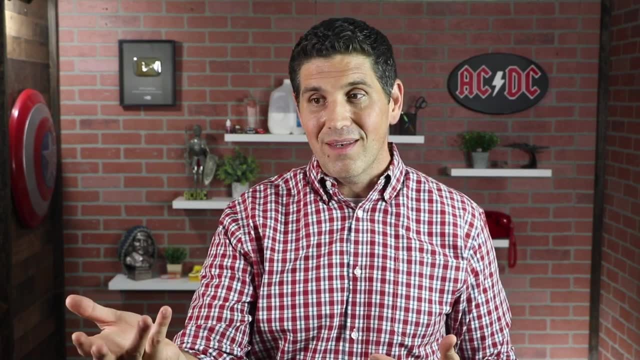 a perfect score in the class if he did Weird. So now what should I do? Because there might be some unforeseen costs. So if I go with the market solution and sell this student my hair, then he's not really gonna learn economics. 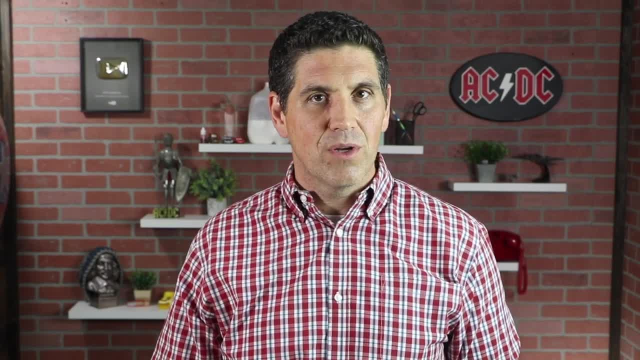 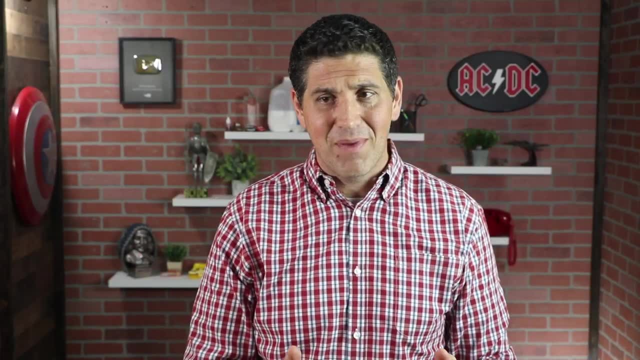 In fact, the only thing he's gonna learn is how to get around and cheat the system, which sounds to me like the making of a serial killer. that would definitely frame me for murder, And never mind the fact that the teacher would probably get fired for this. 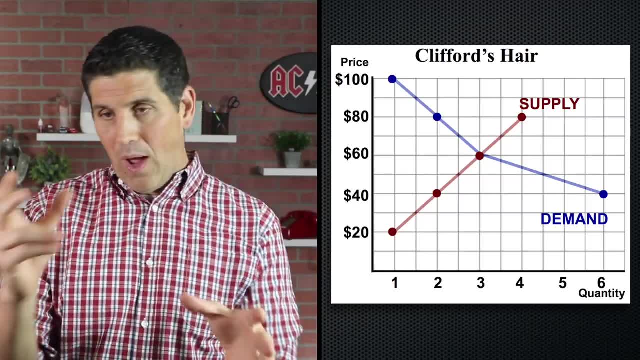 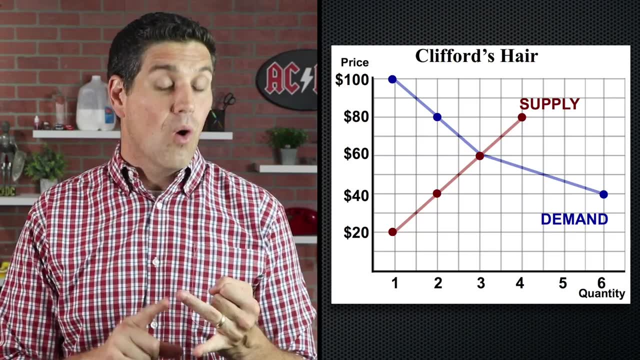 because, let's be honest, it's so against the rules. So now I have to decide: do I want a market that's efficient or do I want to be ethical? And that's exactly why sometimes markets need to be regulated or abandoned, For example, human organs, like the market for kidneys. 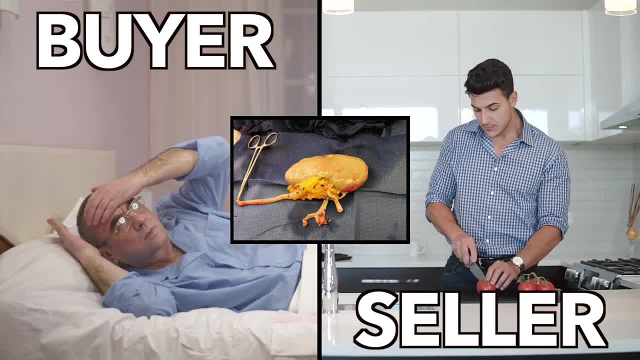 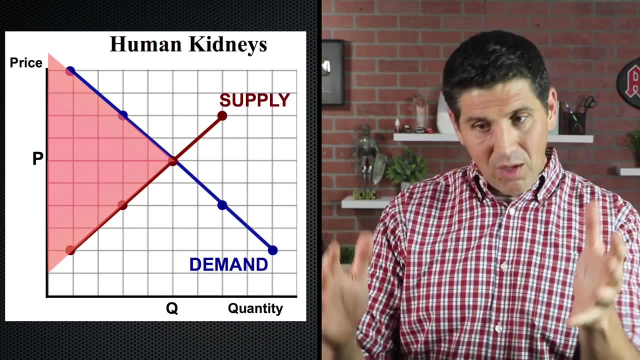 A free market purist would point out. there's people out there that are on dialysis that really want a kidney and there's healthy people out there that, at the right price, are willing to sell a kidney. They would argue that a market would maximize total surplus. 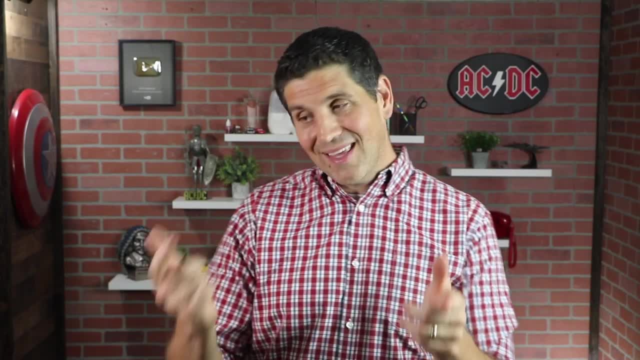 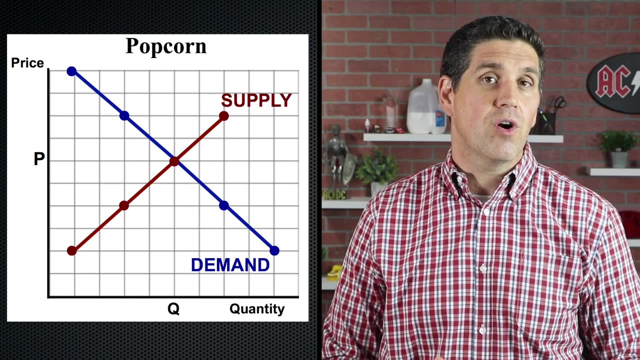 and result in the most efficient outcome. But there's a solid argument against selling kidneys for ethical reasons. But let me point out this is not the norm. In the vast majority of cases, it's the preferred way to allocate our resources, But is it what I should do here in this situation? 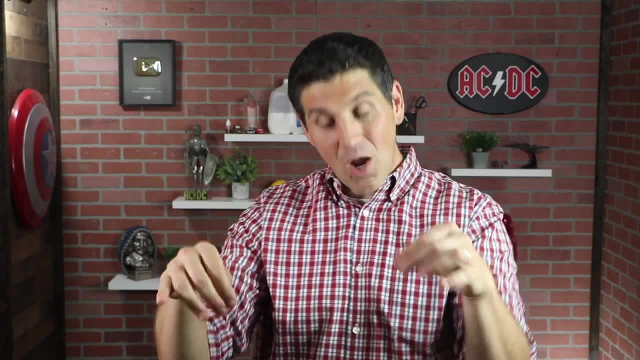 with this guy that wants my hair. I'm gonna let my viewers decide. So let me know in the comments if you think I should give him my hair or sell him my hair, or if I shouldn't do any of that. I wanna know what you think. 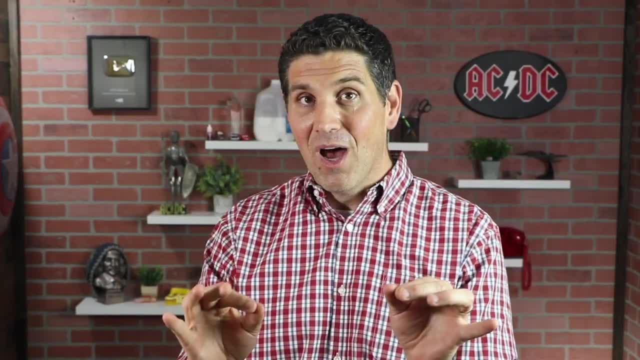 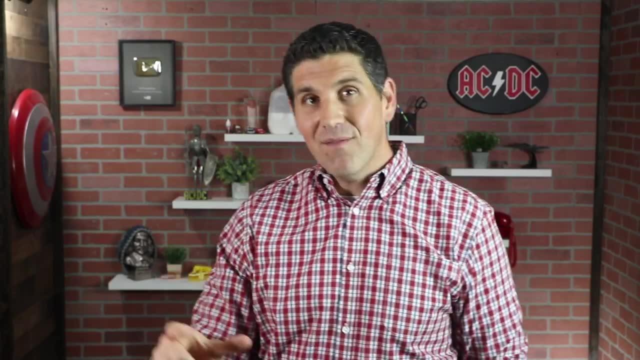 because I don't wanna be considered a sellout. But don't go anywhere because it's time for a pop quiz. Before I do that, let me give you the memory tool that's gonna go on the back wall for this episode. Well, actually there's gonna be two of them. 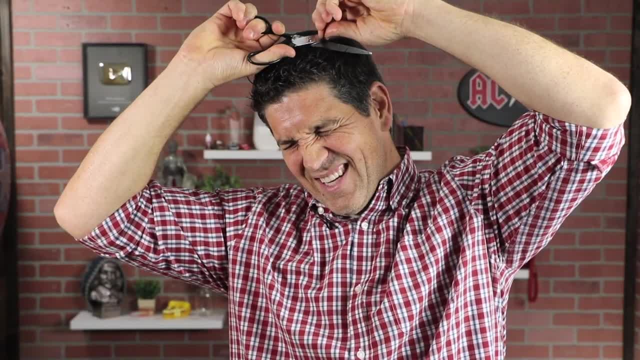 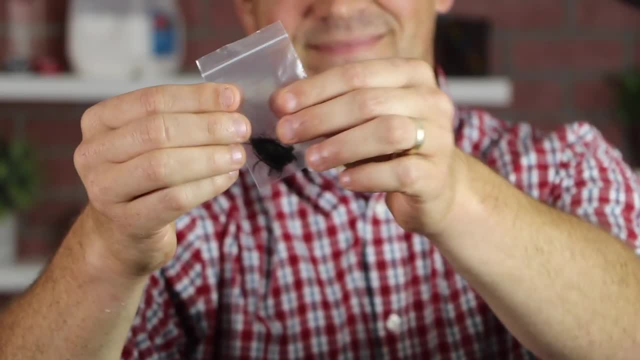 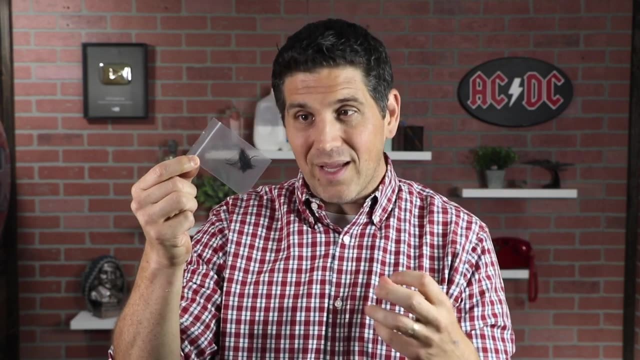 The first one. I need some scissors for Horrible scissors for this. Oh boy, A lock of my hair. This right here is gonna remind you about markets and efficiency and consumer and producer surplus and the whole idea that a demand curve is made up of individuals and their willingness to buy. 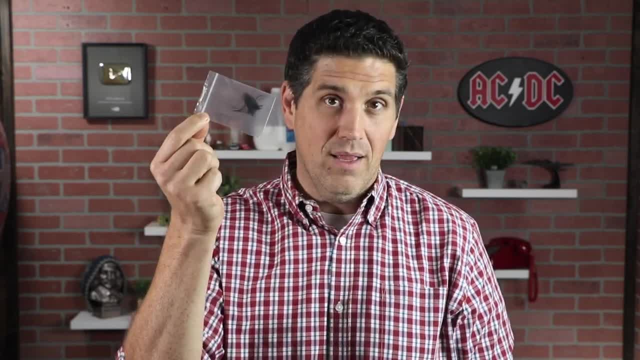 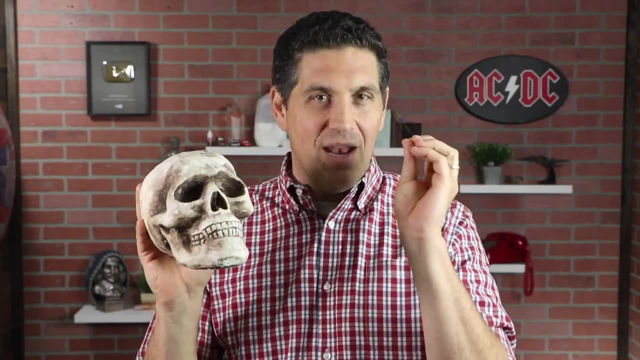 and a supply curve is made up of individuals and their willingness to sell, And the other one is going to be this right here. This represents the idea of dead weight loss and inefficiency and the idea that when a marketer, a market's not producing what it's supposed to produce, 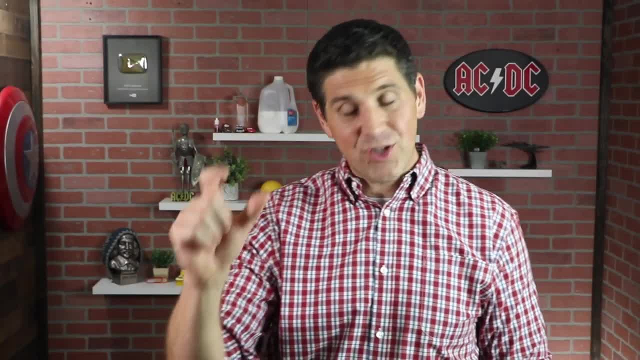 you get dead weight loss. Now I'm gonna give you the quiz. Keep in mind that the questions won't be on the screen for very long, so you have to pause the video. answer the question then. look in the comments below for the answer key. 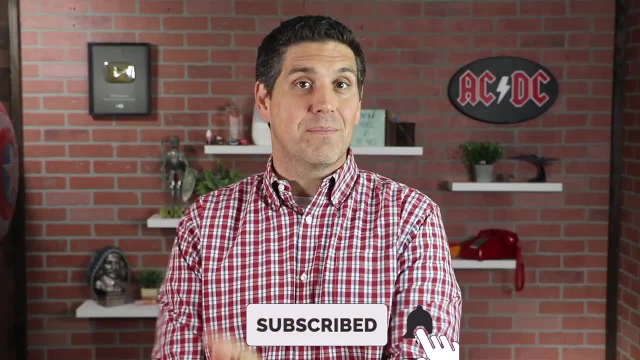 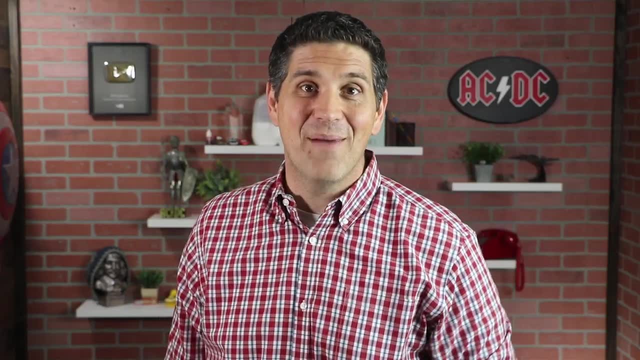 And if you like my videos and they're helping you learn and love economics, please like and subscribe and also check out my ultimate review packet. It's gonna help you learn and do awesome in your class. Thanks for watching, Until next time. Bye. 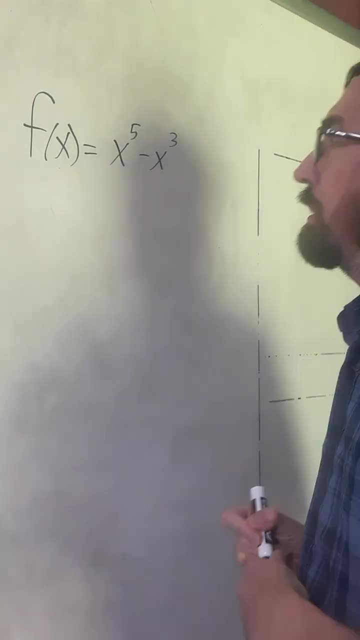 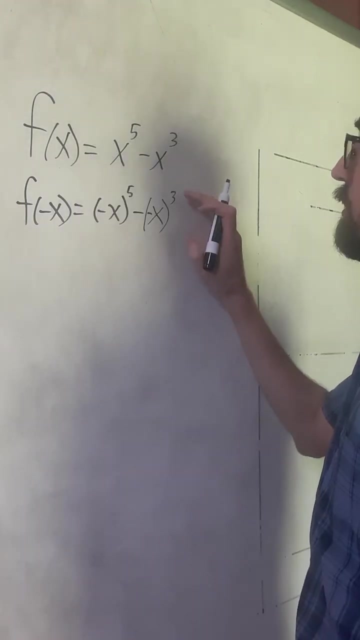 I want to look at this function and determine its symmetry. The first test that we have to do is we need to insert negative x in for every x and see if it matches the original. If that is the case, then we have an even function. If we do this enough times, we will notice that there's a 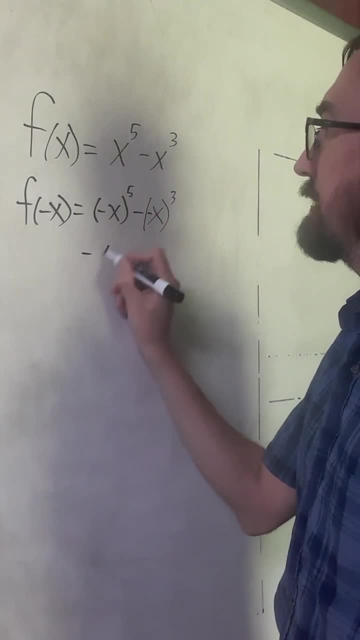 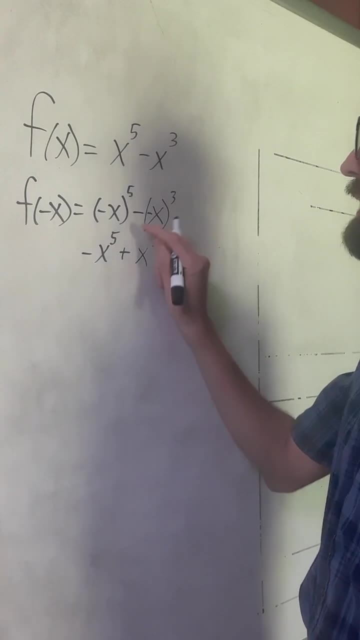 pattern that the odd numbers. they retain their negatives. So this will come back to negative x to the fifth power plus x to the third power. The double negatives make the positive here, And this is what f of negative x is. We notice that these do not match, so we can conclude not. 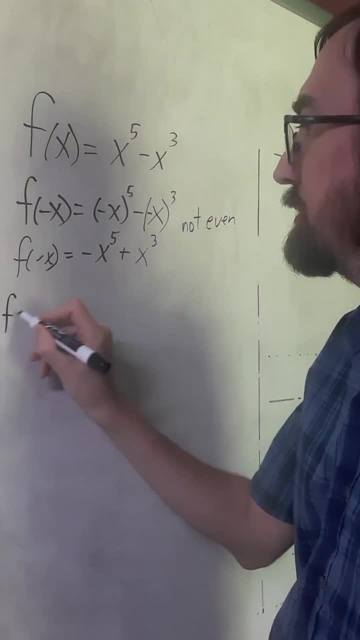 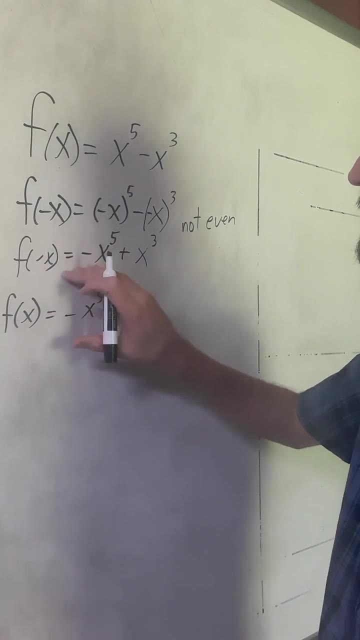 even. The next test we want to do is: we want to do negative f of x. So take the original and multiply through by a negative. Compare this to the f of negative x. They do match. We conclude that this is an even function. If we do this enough times, we can conclude that there's a pattern that the 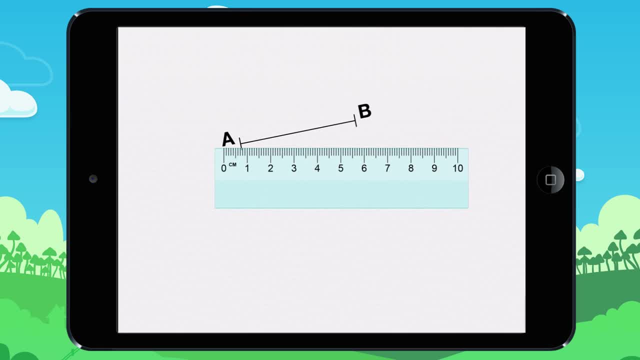 You are going to learn how to measure a line segment. Look, you need to move the ruler. A zero needs to line up with the beginning of the line segment. Now you can measure the length. It is 5 centimeters long. Now you measure the length of the line segment. When you raise a ruler, it will movimento along theively along the long edge. You will also begin to adjust the line segment as you Hierarchy�� lapsionen. Finally, Motta will roll the ruler around the length of a roughly round keepout.